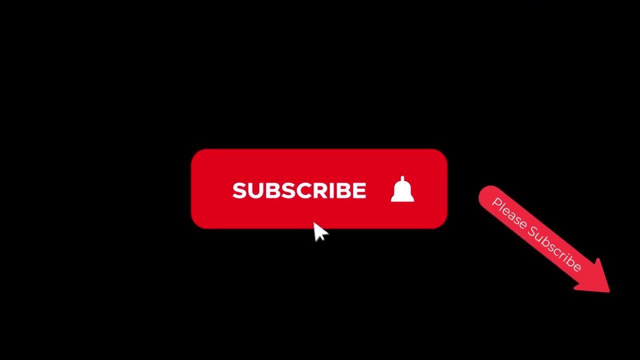 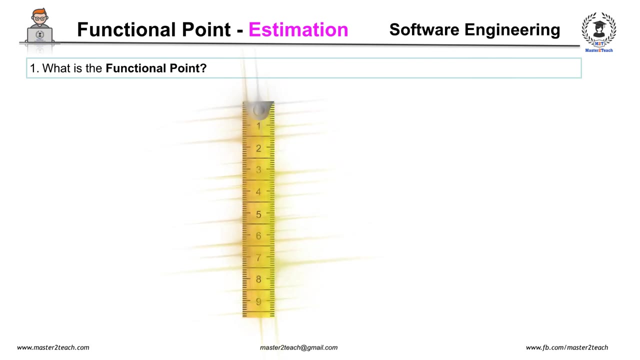 I will try my best to explain step-by-step. If you haven't subscribed to our channel, please click on the subscribe button and subscribe to our YouTube channel. It's really difficult to weight the real values or worth of software. One of the best way. 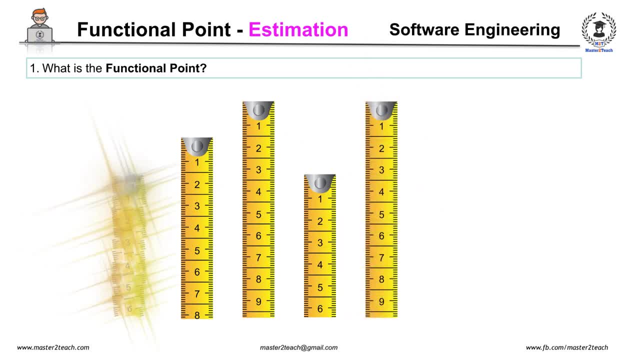 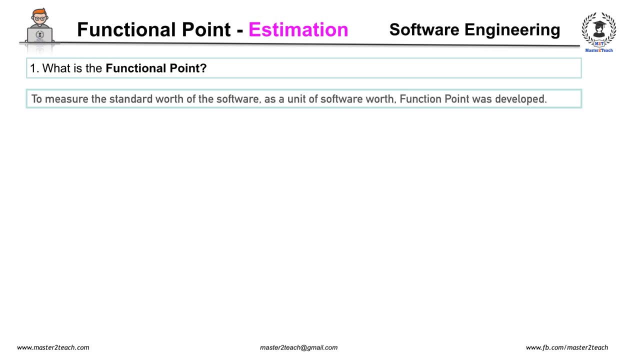 to estimate the software development cost and time is based on the previous software development experience. To measure the standard worth of the software as a unit of software, word functional point was developed. Functional point was first defined by Allen of IBM in 1977. It is used effectively as a means for measuring the functionality delivered by a. 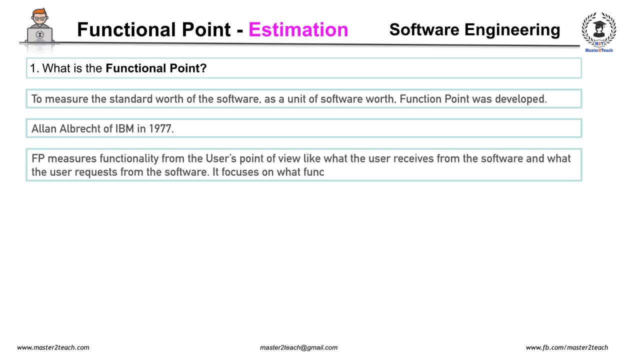 system. Functional point measures functionality from the user's point of view, like what the user receives from the software and what the user requests for the software. It focuses on what functionality is being delivered. According to the wiki, a functional point is a unit of measurement to express the amount of business functionality and information. 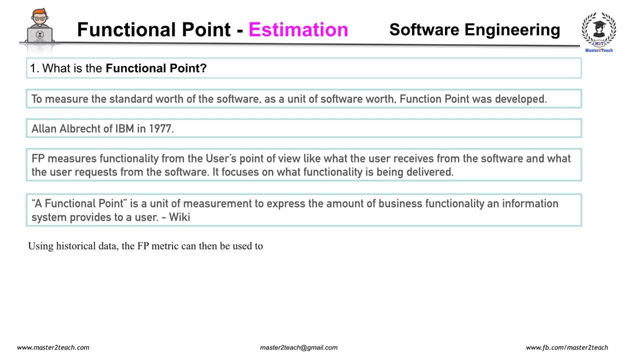 system provided to a user Using historical data. the functional point matrix can then be used to estimate the cost or effort required to design, code and test the software. Predict the number of errors that will be encountered during testing. Forecast the number of components. 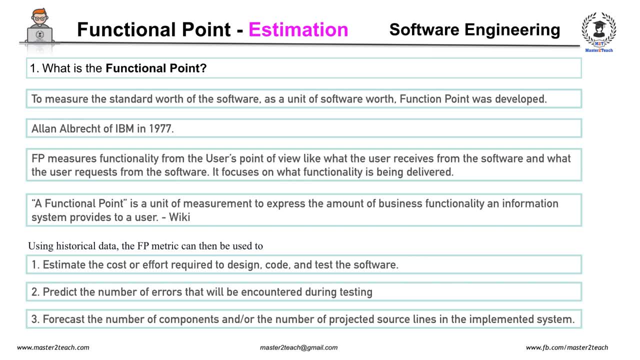 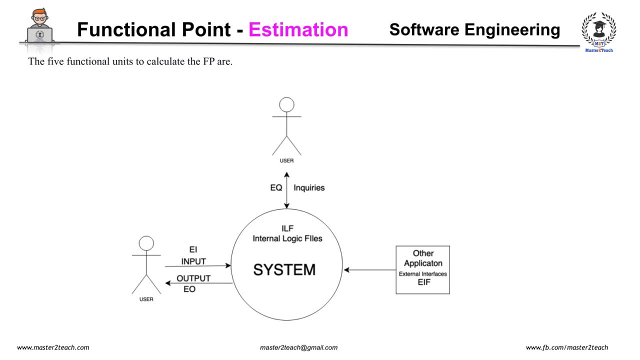 and or the number of projected source lines in the implemented system. Functional points are derived using an empirical model. The functional points are derived using an empirical relationship based on the countable measure of software information domains and the qualitative assessment of the software complexity. The five functional units which are considered information domains as input to calculate. 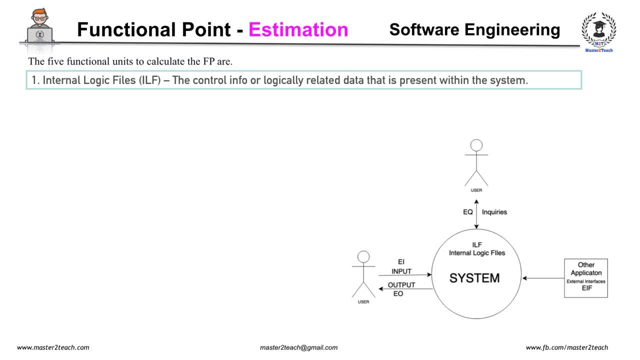 the functional point are: Internal Logic files, The Controlled input or logically related data that is present within the system. External interface files, The controlled data or other logical data referred by the system but presence in another system. External input data or control input that comes from outside our system. External output: data that goes out of the system after. 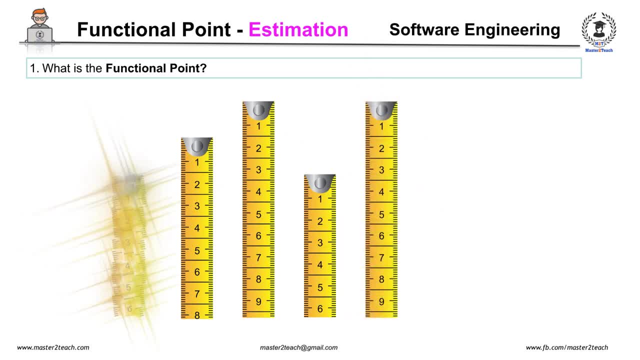 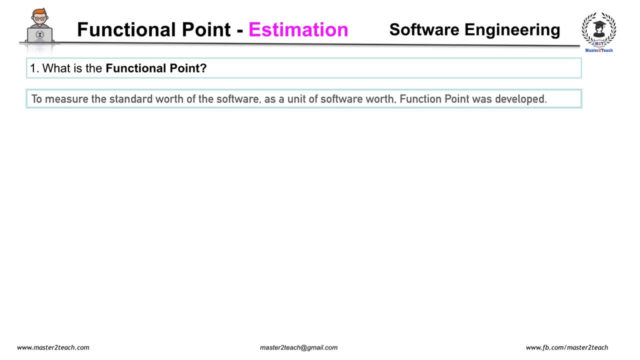 to estimate the software development cost and time is based on the previous software development experience. To measure the standard worth of the software as a unit of software, word functional point was developed. Functional point was first defined by Allen of IBM in 1977. It is used effectively as a means for measuring the functionality delivered by a. 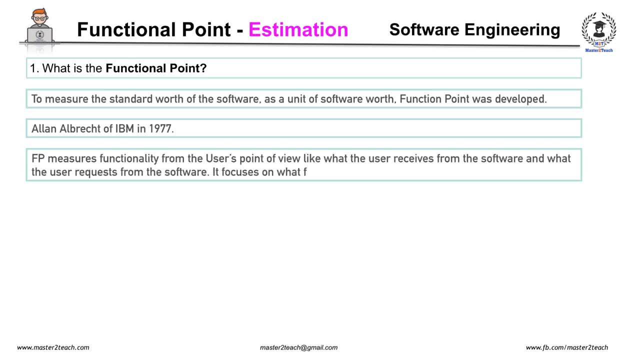 system. Functional point measures functionality from the user's point of view, like what the user receives from the software and what the user requests for the software. It focuses on what functionality is being delivered. According to the wiki, a functional point is a unit of measurement to express the functionality of the software. 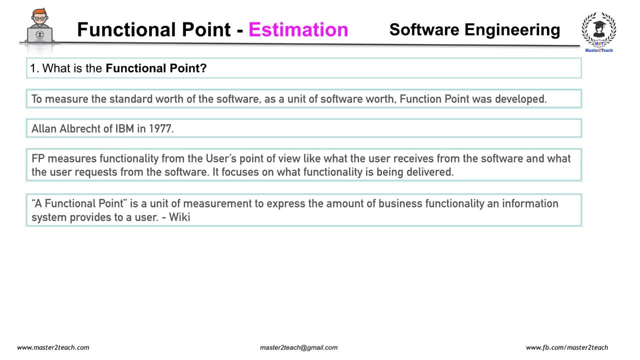 This will test the amount of business functionality and information this system provides to the user. Using historical data, the functional point matric can then be used to estimate the cost or effort required to design, code and test the software. Predict the number of errors that will be encountered during testing. Forecast the number. 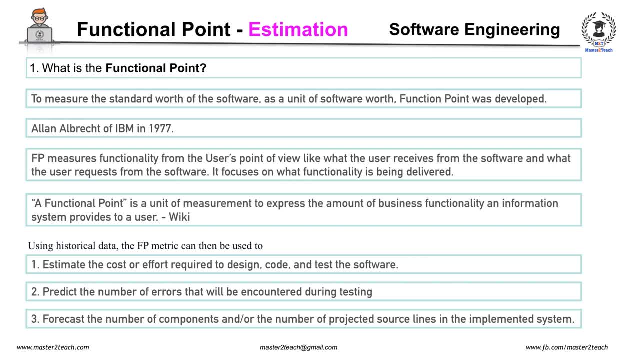 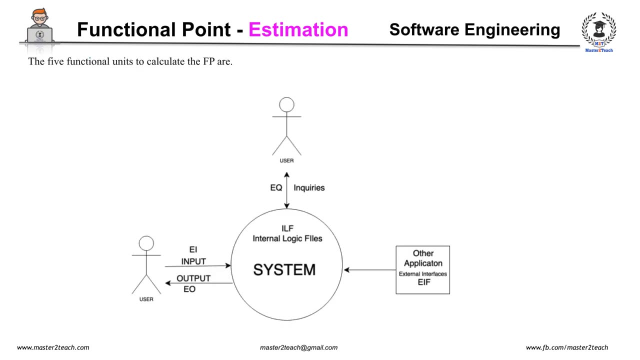 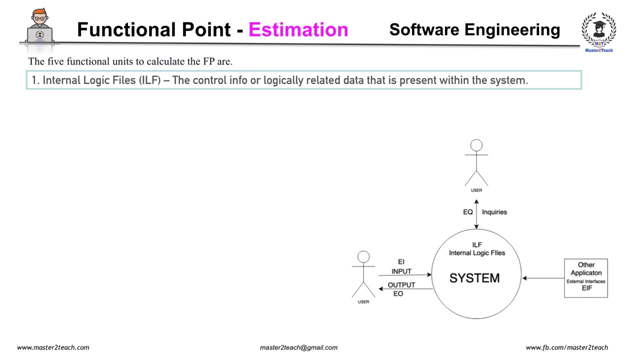 of components and or the number of projected source lines in the implemented system. Functional points are derived using an empirical relationship based on countable measures of software information domains and qualitative assessments of software complexity. the five functional unit which is considered information domains as input to calculate the functional point are: internal logic files, ILF. 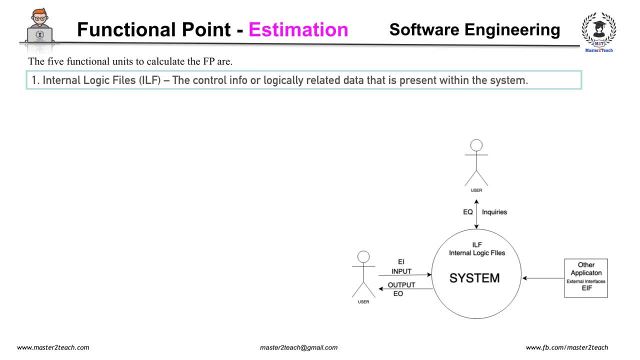 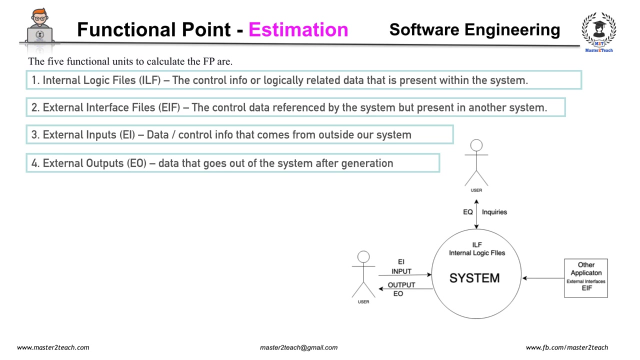 the control info or logically related data that is present within the system. external interface files, EIF, the control data or other logical data referred by the system but presents in another system. external input data or control info that comes from outside our system. external output data that goes out of the system after generation. external inquiries. combination of input. 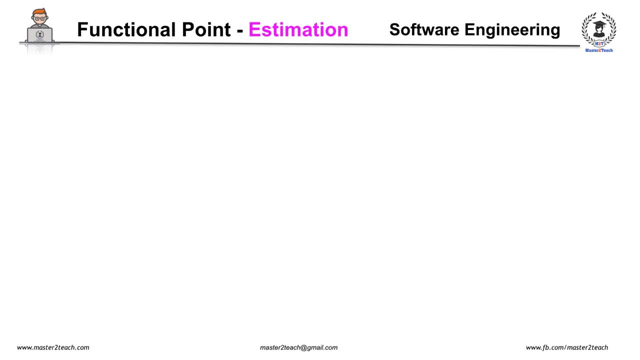 and output, resulting data retrieval. now let's move to calculate functional point. to calculate functional point, the functional relationship is used. functional point is called to UFP into CAF, where UFP is unadjusted functional point and CAF is complexity adjustment factor. let's follow step by step, step one, calculating unadjusted functional point. 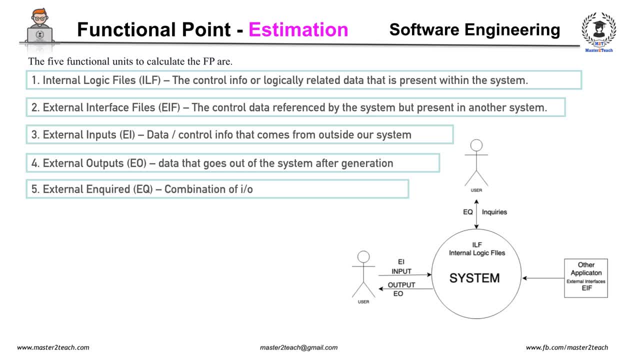 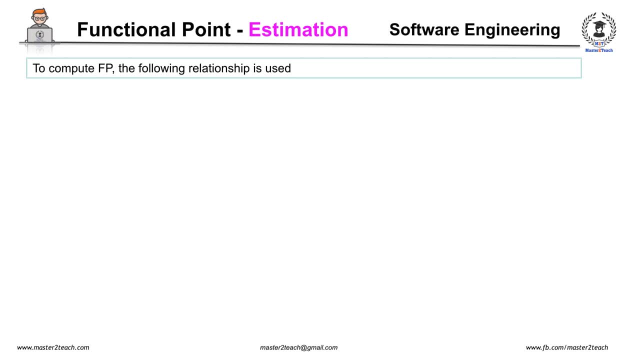 generation, External inquiries, combination of input and output, resulting data retrieval. Now let's move to calculate functional point. To calculate functional point, the functional relationship is used. Functional point is called to UFP into CAF, where UFP is unadjusted functional point and CAF is complexity. 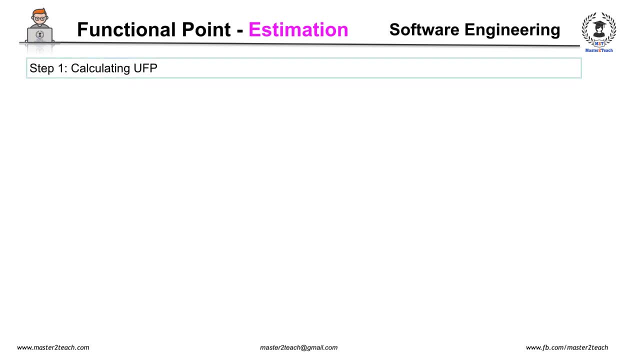 adjustment factor. Let's follow step by step, Step 1, calculating unadjusted functional point. Each functional point is ranked according to complexity. There exists predefined weights for the each functional point in each category. Organization that use functional point methods develop criteria for determining. 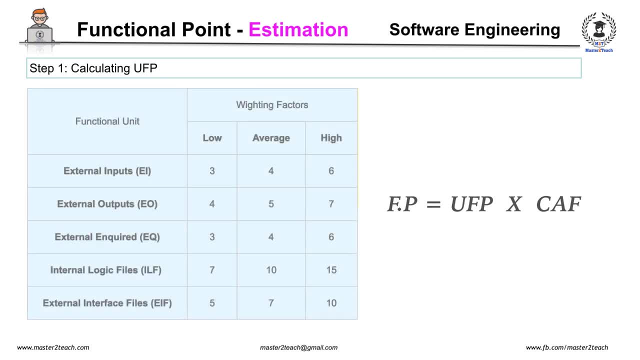 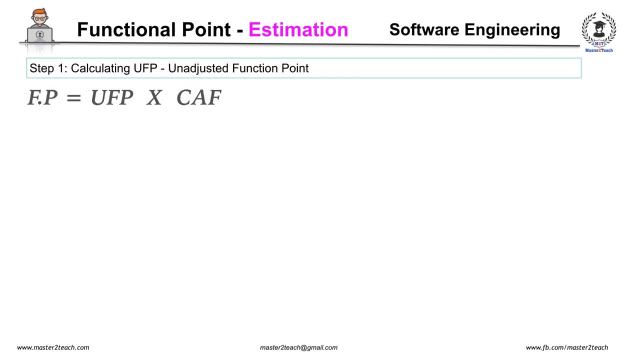 whether a particular entry is simple, average or complex. Now let's see how it works. Nonetheless, the determinations of complexity is somewhat subjective. Unadjusted functional point is called to sum of all the complexity of the EI, EOs, EQs, ILFs. 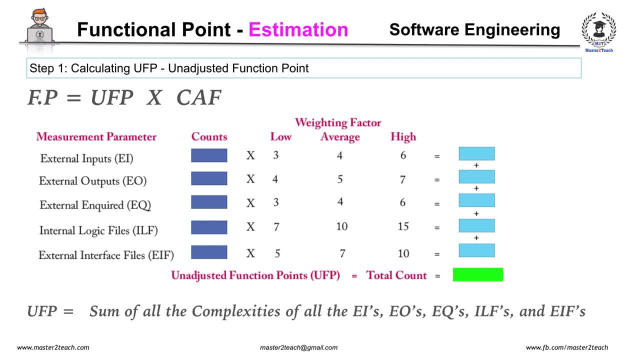 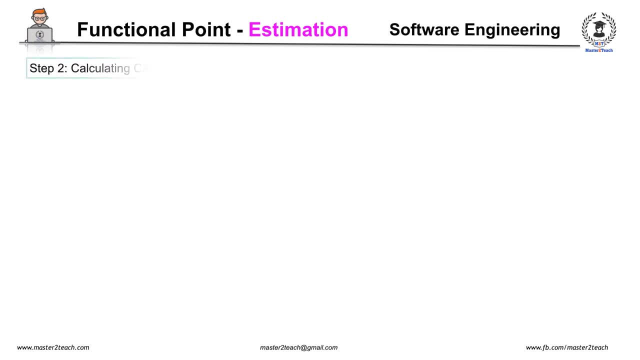 and EIFs: External inputs, external outputs, external inquiries, external interface files and internal logic files. Step 2, calculating CAF complexity adjustment factor. Complexity adjustment factor. as we know, complexity adjustment factor is called to 0.65 plus 0.01 into summation EFI, where: 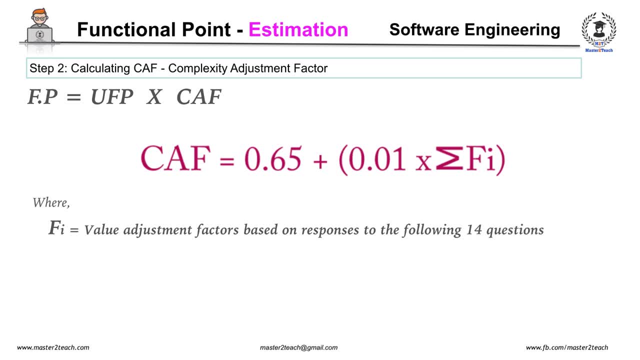 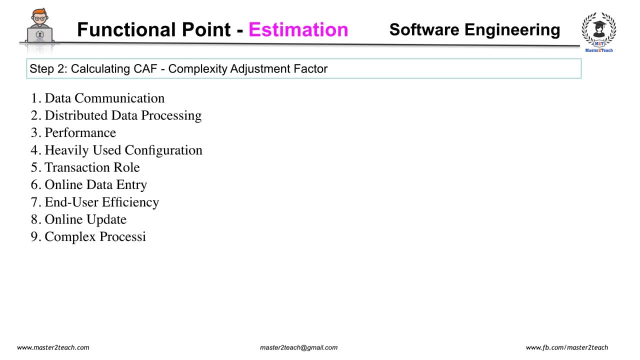 EFI is value adjustment factor Based on responses to the following 14 question. Complexity adjustment factor is calculated using 14 aspects of processing complexity and these 14 questions answer on the scale of 0 to 5.. means no influence or no impotence. one mean incidental, two mean moderate, three: 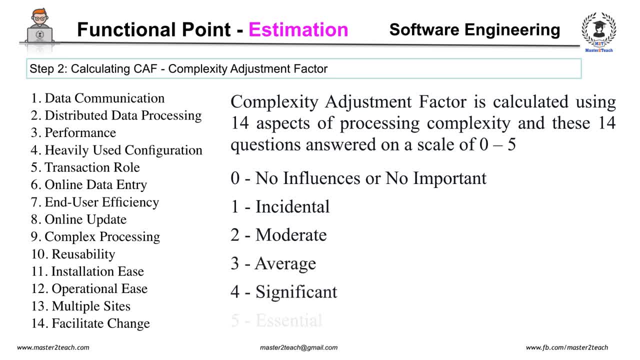 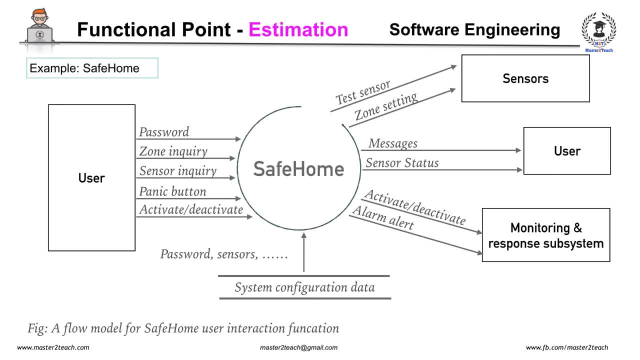 mean average, four mean significant, five mean essential. to illustrate the use of functional point matrix, let's see a simple analysis model: safe home. the function manages user interaction, accepting a user password to activate or deactivate the system and allows inquiries on the status of security zones and various security sensor. the function displays a series of prompting. 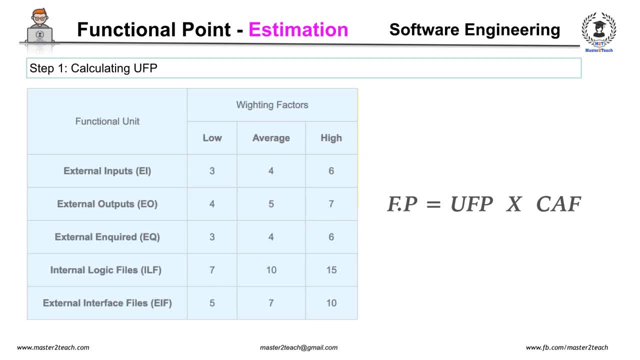 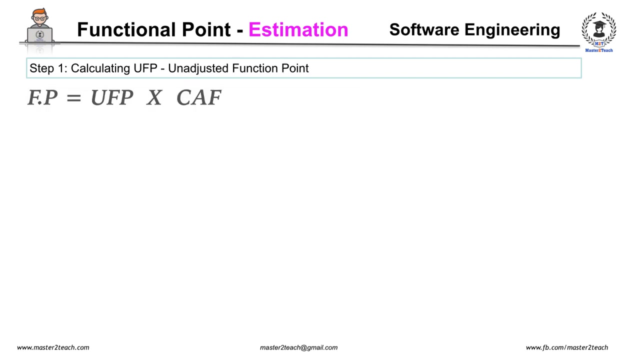 each functional point is ranked according to complexity. there exists predefined weights for the each functional point in each category. organization that use functional point methods develop criteria for determining whether a particular entry is simple, average or complex. nonetheless, the determination of complexity is somewhat subjective. unadjusted functional point is called. 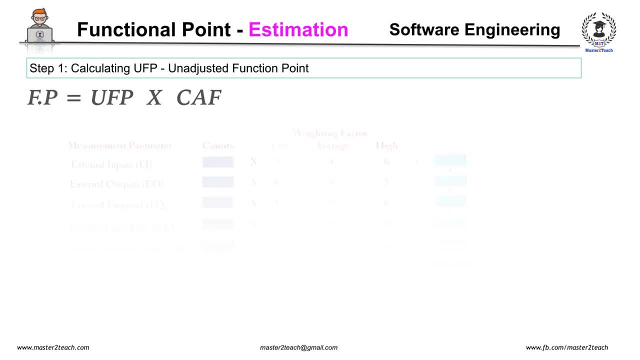 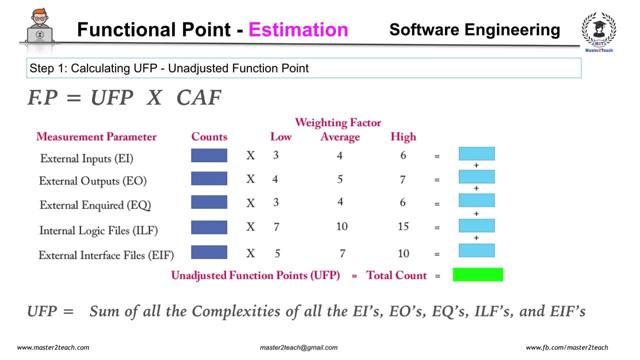 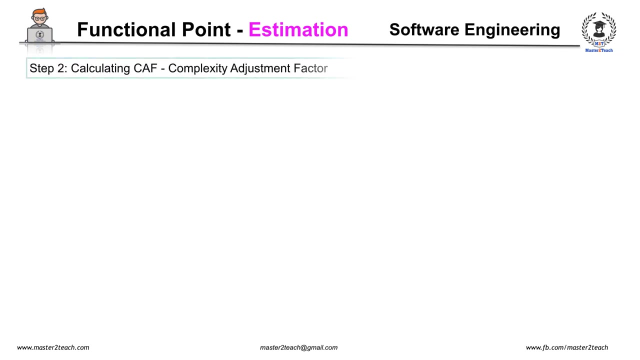 to sum up all the complexity, after EI, EO's, EQ's, ILF's and EIF actually inputs, external outputs, externally inquiries, external interim race files and internal logic files, is step to calculating CAF complexity adjustment factor. complexity adjustment factor. as we know, complexity adjustment factor is called the CAF orив. CAF. complexity adjustment factor is qua in ICPC of multiple levels, a complex rate Healthcare recipe, recipe recipe ways foről CAFancof complexity compensation practice term one, and that means CAF and the EAF answer to the future of complexity conditions. связemat goin to all. the Pfimod EII tastes coolям. 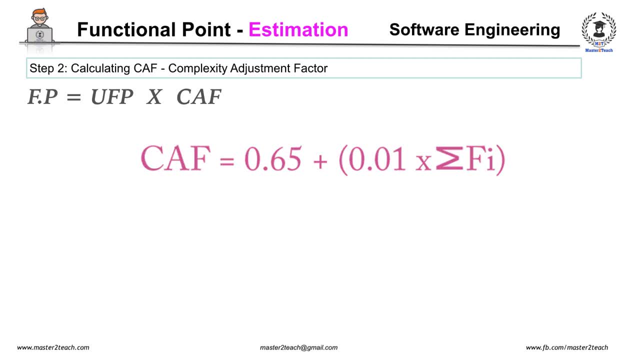 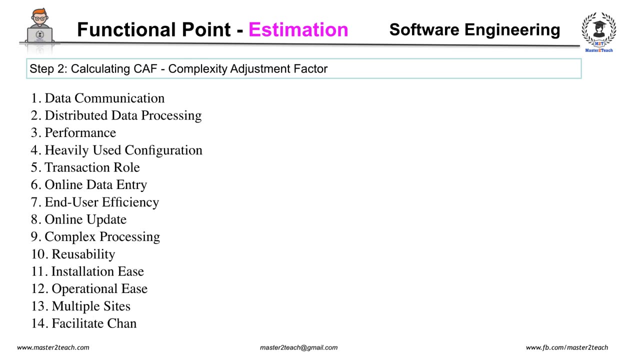 equal to 0.65 plus 0.01 into summation Fi, where Fi is value adjustment factor based on responses to the following 14 questions. complexity adjustment factor is calculated using 14 aspects of processing complexity and these 14 questions answer on the scale of 0 to 5. 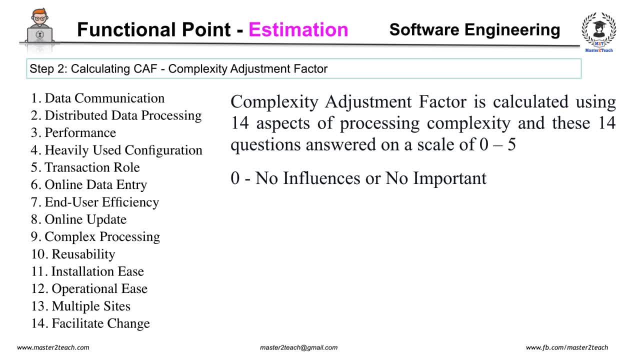 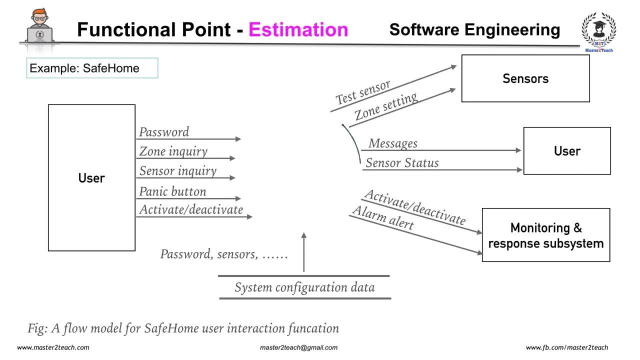 zero means no influence or no impotence, one mean incidental, two mean moderate, three mean average, four mean significant, five mean essential. to illustrate the use of functional point matrix, let's see a simple analysis model: safe home- the function manages user interaction, accepting a user password to activate or 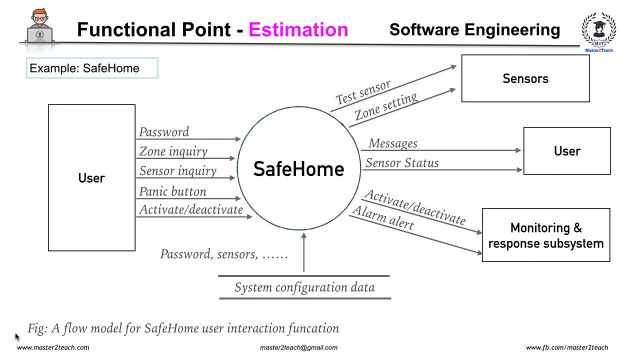 deactivate the system and allows inquiries on the status of security zones and very security sensor. the function displays a series of prompting messages and sends appropriate control signals to various components of the security system. the data flow diagram is evaluated to determine a set of the key information domain measures required for computations of the function point. 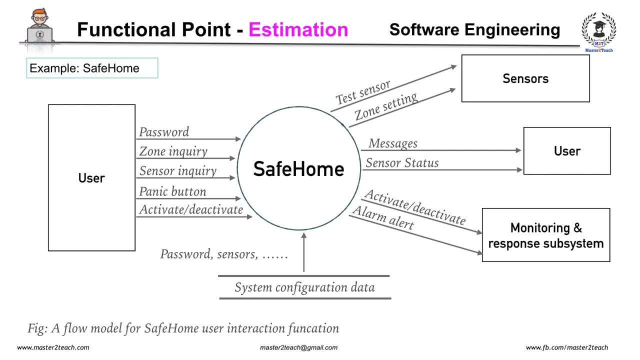 messages and sends appropriate control signals to various components of the security system. the data flow diagram is evaluated to determine a set of the key information domain measures required for computations of the function point matrix. three external inputs: password, panic button and activate or deactivate. two external inquiries: zone inquiry and sensor inquiry. one ILF system configuration file, two external. 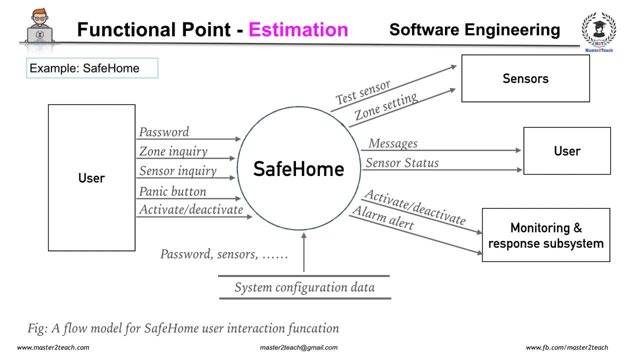 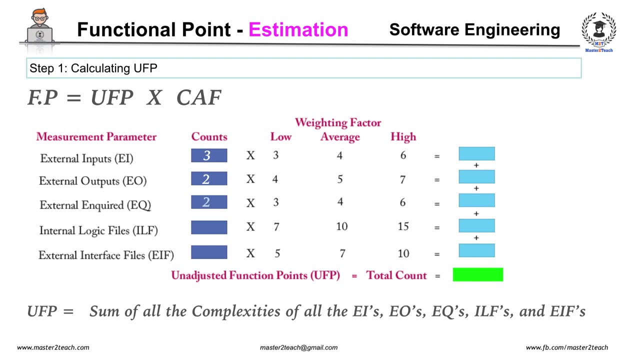 input messages and sensor status. and four EIF test: sensor zone setting, activate, deactivate and alarm alert. now calculating unadjusted functional point with the simple weighting factor. therefore, UFP, unadjusted function point, is equal to 50. now moving to calculate. now moving to calculate CAF. as we know, CAF is equal to 0.65 plus 0.01 into. 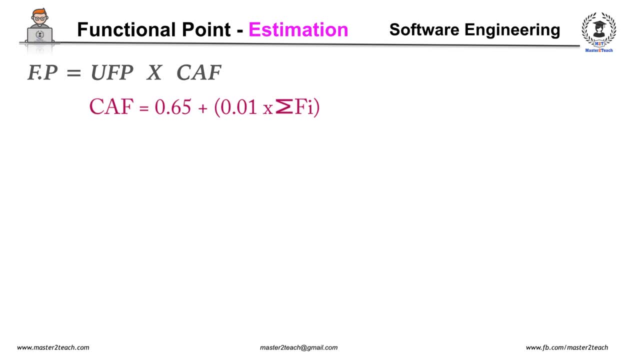 summation f i. let's calculate in a moderately complex product. then summation f i is called to 14 into 2, is called to 28, because all the 14 questions are answered in the moderate form, which is equal to 2, which is 1.5, as we know. if 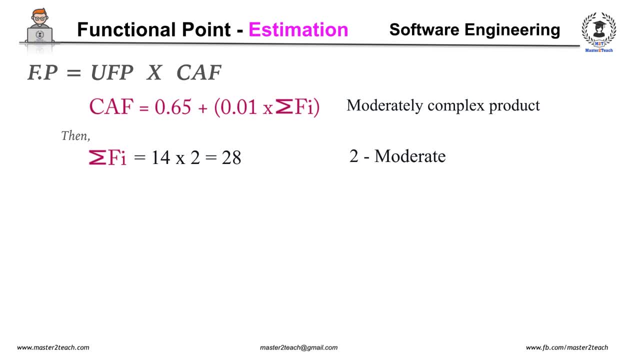 if the answer is correct, in to 2, so that 14 into 2 is equal to 28, CF is equal to 0.93. as we know, functional point is equal to UFP into CAF. unadjusted functional point is equal to 50 and CF is equal to 0.93. therefore, functional point is equal to. 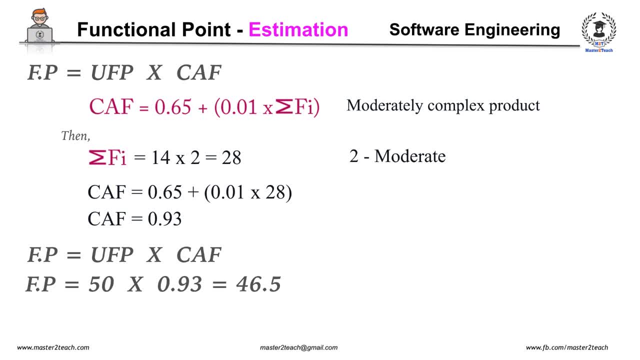 46.5. based on the projected functional point values derived from the requirement model, the project team can estimate the overall implemented size of the safe home user interaction function. assume that past data indicates that one functional point translate into 60 lines of code and that 12 function points are. 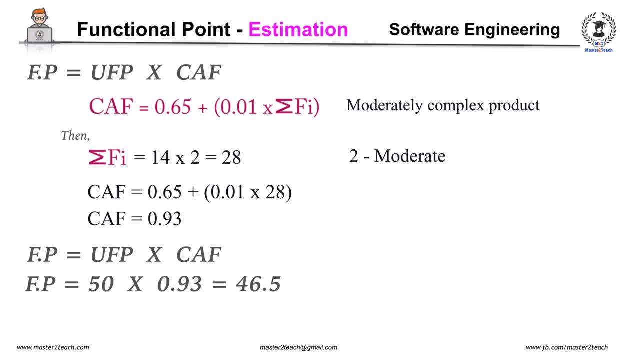 produced for each person month of report. this historical data provides the project manager with important planning information that is based on the requirements model rather than preliminary estimates. assume further that past projects have found an average of 3 rows performance function point during requirements and design review and 4 errors per functional point during. 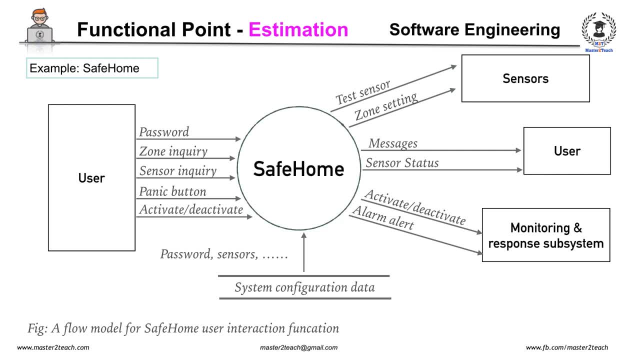 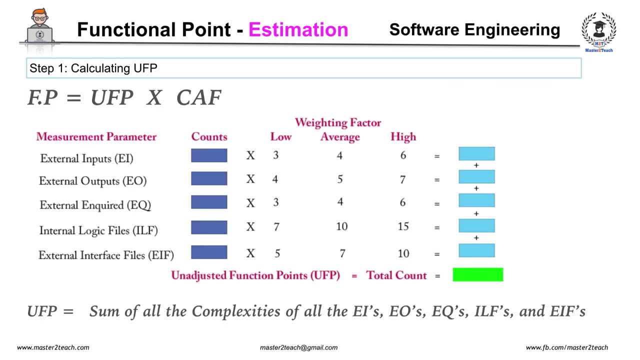 matrix: three external inputs, password, panic button and activate or deactivate, two external inquiries- zone inquiry and sensor inquiry, one ILF system configuration file, two external input messages and sensor status and four EI of test: sensor zone setting, activate, deactivate and alarm alert. now calculating unadjusted functional point with the simple weighting factor. 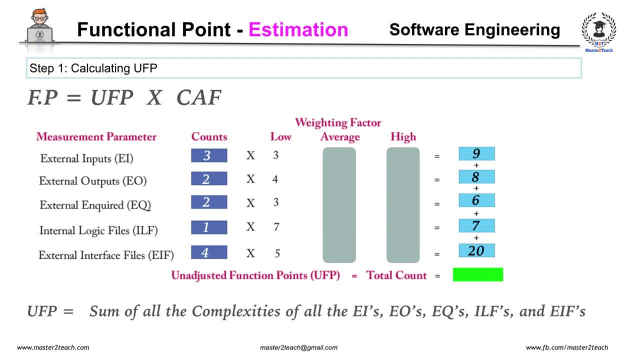 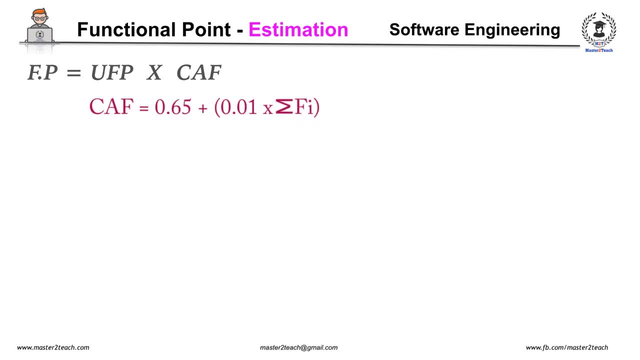 therefore UFP, unadjusted functional point, is equal to 50. now moving to calculate CAF. as we know, CF is called 0.65 plus 0.01 into summation FBI. let's calculate in a moderately complex product. then summation, if I is called to 14 into 2, is called to 28 because all the 14 questions. 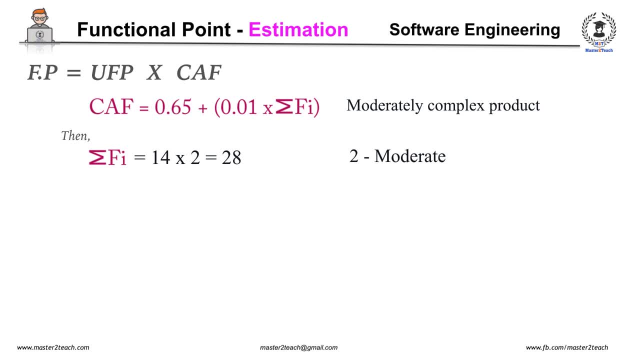 are answered in the moderate form, which is equal to 2. so that's a quick summary of his answers in the moderate form, which is equal to 2. so that's a quick summary of his answers. answers are. answers are answered in the moderate form, which is equal to 2. so that's a quick summary of his. 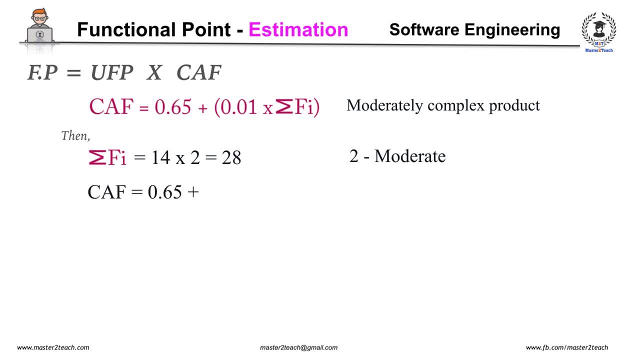 that 14 into 2 is equal to 28, cf is equal to 0.93. as we know, functional point is equal to uefp into caf, unadjusted, functional point is equal to 50 and cf is equal to 0.93, therefore functional. 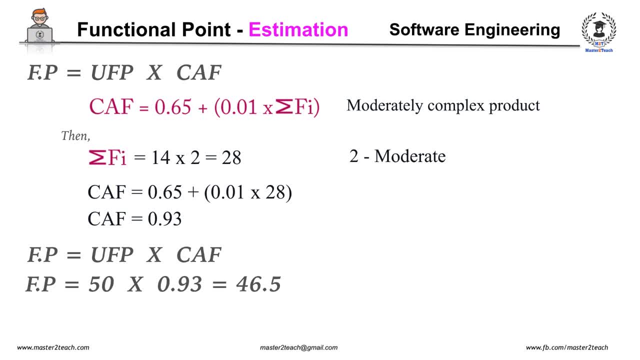 point is equal to 46.5. based on the projected functional point values derived from the requirement model, the project team can estimate the overall implemented size of the safe home user interaction function. assume that past data indicates that one functional point translate into 60 lines of code and that 12 functional points are produced for each person month of. 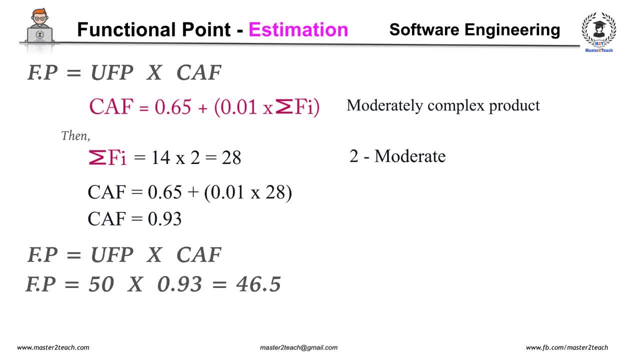 report. this historical data provides the project manager with important planning information that is based on the requirements model rather than preliminary estimates. assume further that past projects have found an average of three errors per function point during requirements and design review and four errors per functional point during the. 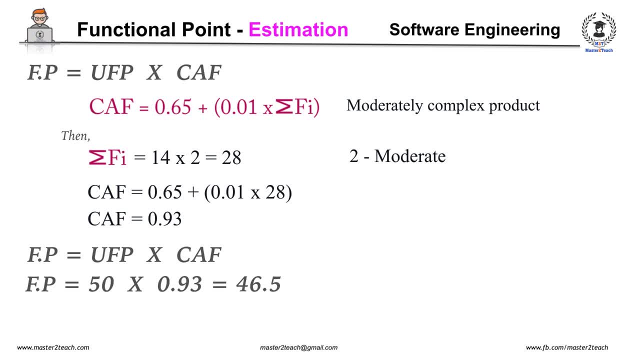 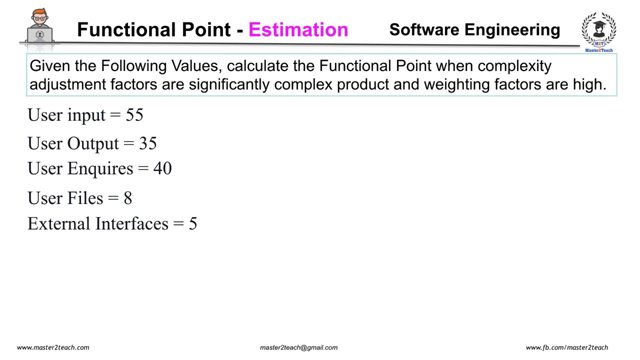 the unit and integration testing. These data can ultimately helps you to assess the completeness of your review and testing activities. Let's see one more example of calculating functional point. Given the functional values, calculate the functional point when complexity, adjustment factor are significantly complex, product and weighting factor are high. 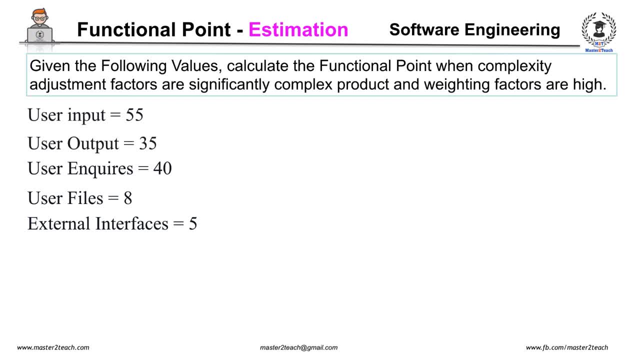 User input is equal to 55,, user output is equal to 35, user inquiry is 40, user files 8, whereas external interface is 5.. We know that functional point is equal to unadjusted functional point. multiplication of CAF complexity adjustment factor where UFP is equal to sum of all the complexities. 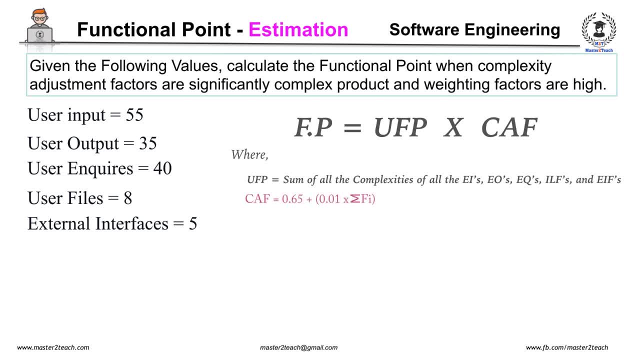 of the 5 input variables and CAF is equal to 0.65 plus 0.0 into summation of 5.. And where summation of 5 is equal to value adjustment factor. Now let's calculate unadjusted functional point. 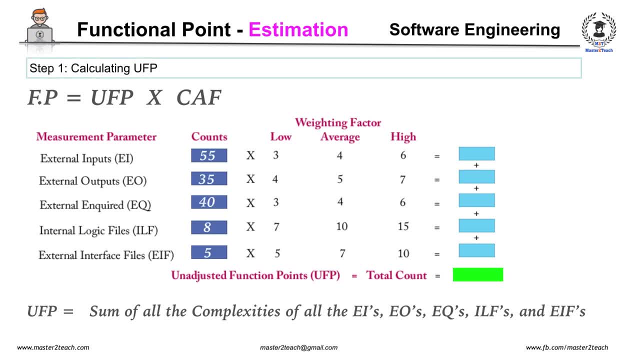 Filling table data. here we are required to calculate in the high weighting factor, so that unadjusted functional point is equal to 330 plus 245 plus 240 plus 120 plus 50, which is equal to 985.. Now moving to calculate CAF complexity adjustment factor. 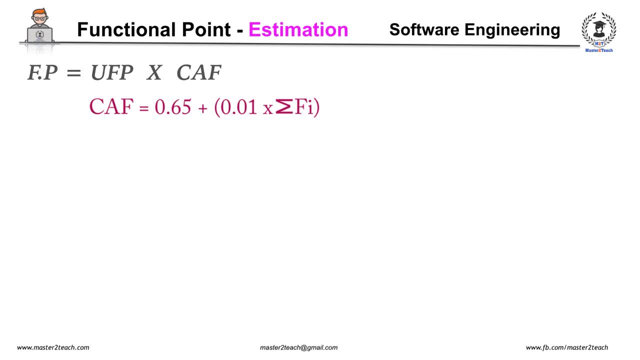 Where F is equal to 0.65 plus 0.01 into summation of 5.. Here we are required to calculate all 14 complexity factors in significantly complex Summation of 5 is equal to 14 into 4 is equal to 56.. 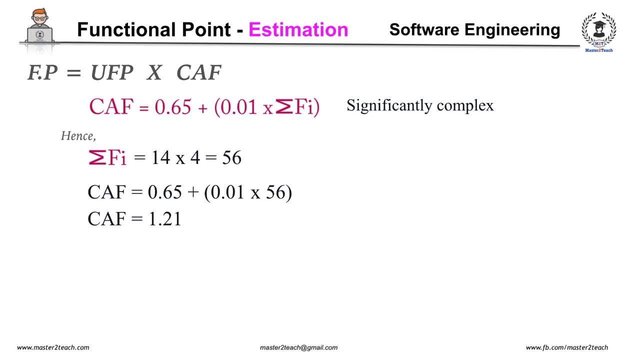 Therefore, CAF is equal to 1.21. What if complexity factor of 5 questions are average, 5 questions are moderate and 4 questions are no influence? Then Summation of 5 is equal to 5 into 3 plus 12.. 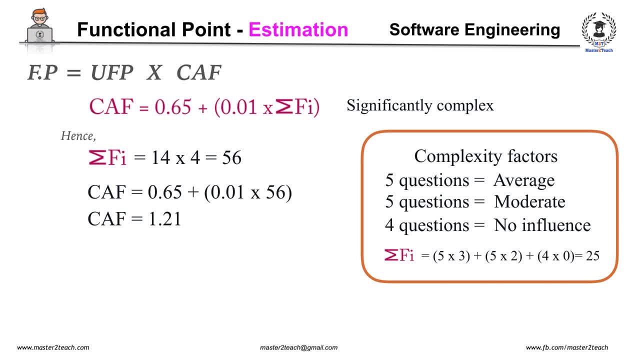 plus 5 into 2, plus 4 into 0 is equal to 25.. Therefore, final functional point is called to UFP into CAF. Unadjusted functional point, multiplication of CAF is complexity adjustment factor. Therefore, functional point is equal to 985 into 1.21, which is equal to 1191.85.. 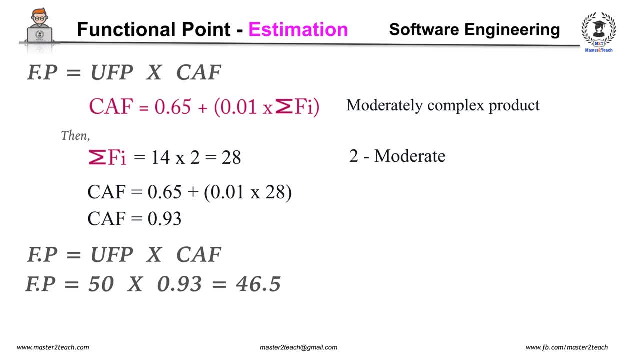 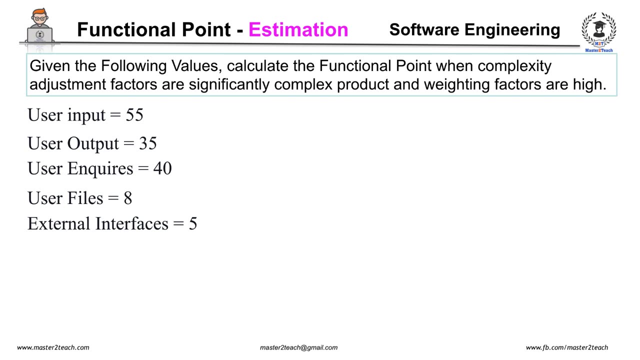 unit and integration testing. this data can ultimately helps you to assess the completeness of your review and testing activities. let's see one more example of calculating functional point. given the functional values, calculate the functional point. when complexity, adjustment factor are significantly complex, product and weighting factor are high, user input is equal. 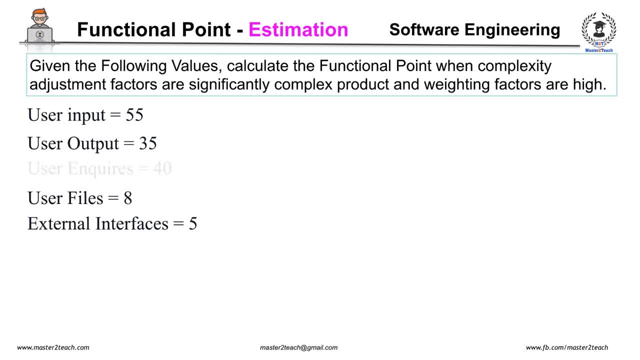 to 35, user output is equal to 35, user inquiry is 40, user files 8, whereas external interfaces 5.. we know that functional point is called unadjusted functional point. multiplication of caf, complexity adjustment factor, where ufp is called sum of all the complexities of the five input variables. 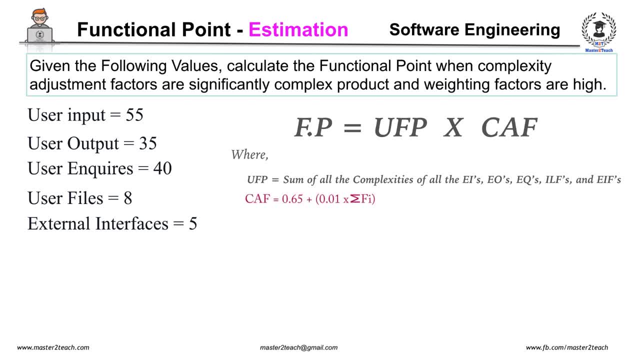 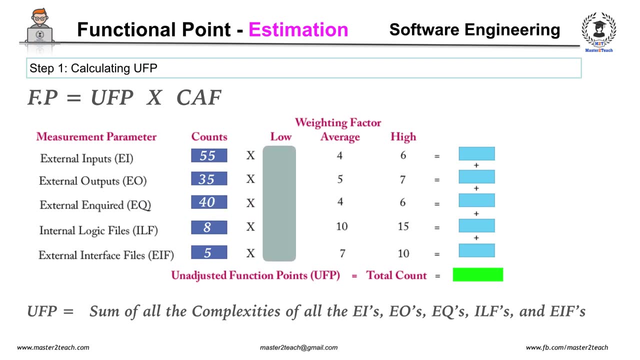 and cf is equal to 0.65 plus 0.0, into summation f i and where summation f i is equal to value adjustment factor. now let's calculate unadjusted functional point filling table data. here we are required to calculate in the high weighting factor, so that 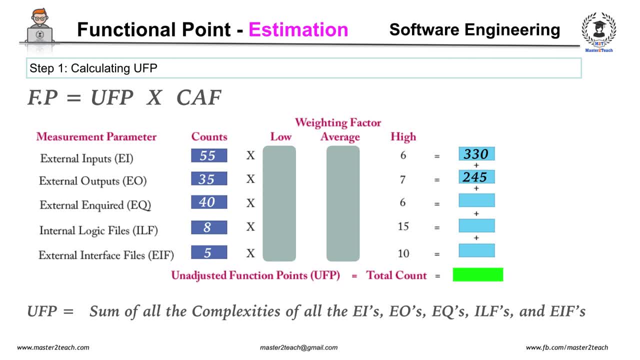 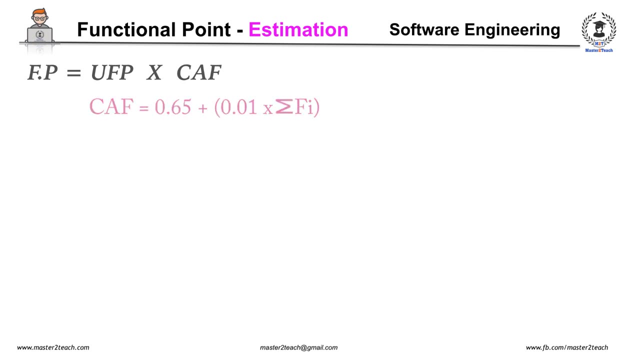 unadjusted functional point is equal to 330 plus 245 plus 240 plus 120 plus 50, which is equal to 985. now moving to calculate caf, complexity adjustment factor cf is equal to 0.65 plus 0.01 into summation f i. here we are required to calculate all 14 complexity factors in. 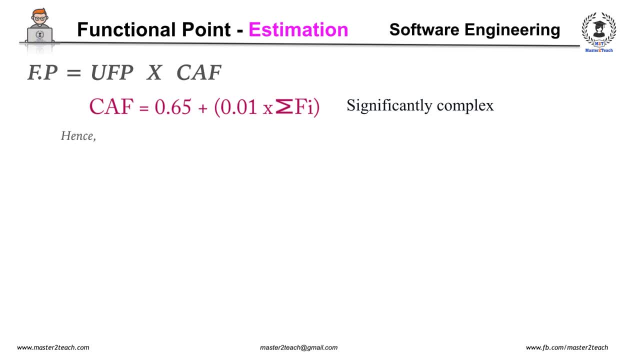 significantly complex. hence summation f i is equal to 14 into 4 is equal to 56. therefore cf is equal to 1.21. what if complexity factor of 5 questions are average, 5 questions are moderate and 4 questions are no influence, then summation f i is equal to 5 into 3 plus 5 into 2 plus. 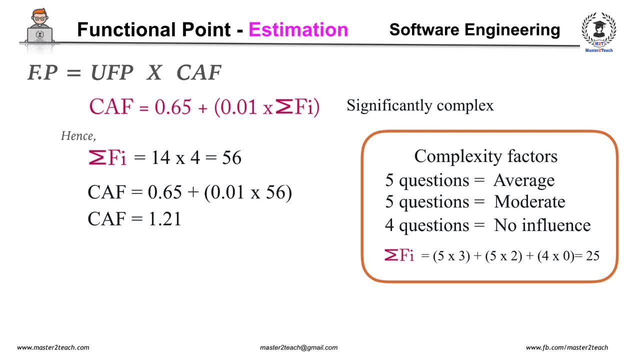 4 into 0 is equal to 25. therefore, final functional point is called to ufp into caf. unadjusted functional point. multiplication of cf is complexity adjustment factor. therefore, functional point is equal to 985 into 1.21, which is equal to 1191.85. in this way we can calculate: